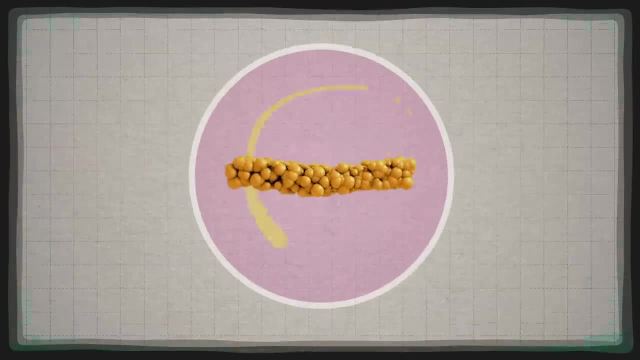 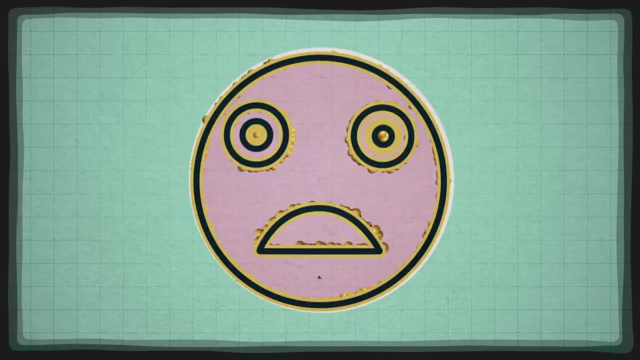 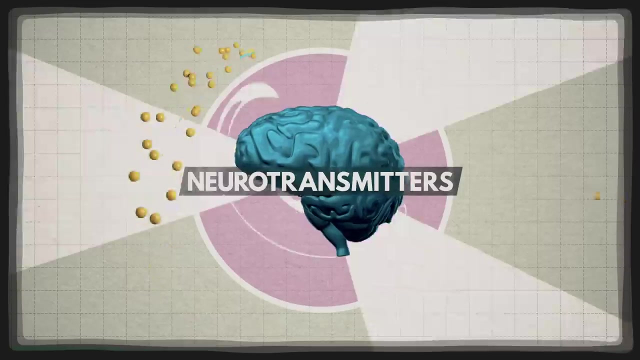 Meanwhile, proteins and amino acids, the building block nutrients of growth and development, manipulate how we feel and behave. Amino acids contain the precursors to neurotransmitters, the chemical messengers that carry signals between neurons, affecting things like mood, sleep, attentiveness and weight. 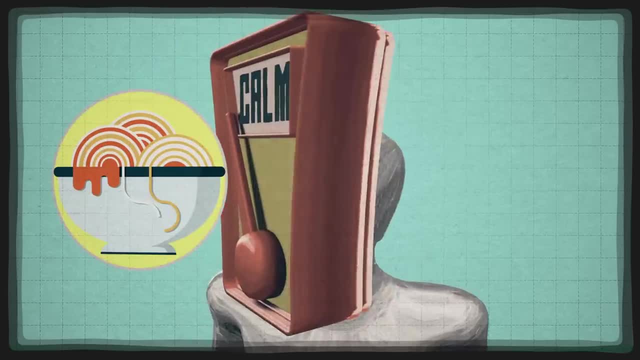 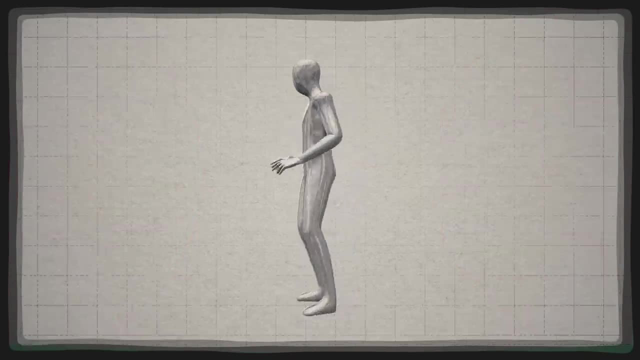 They're one of the reasons we might feel calm after eating a large plate of pasta or more alert after a protein-rich meal. The complex combinations of compounds in food can stimulate brain cells to release mood-altering norepinephrine dopamine. 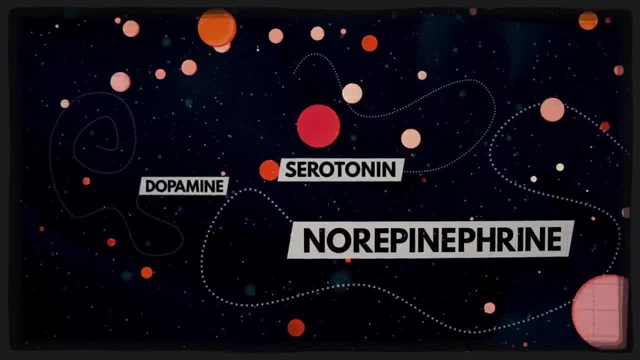 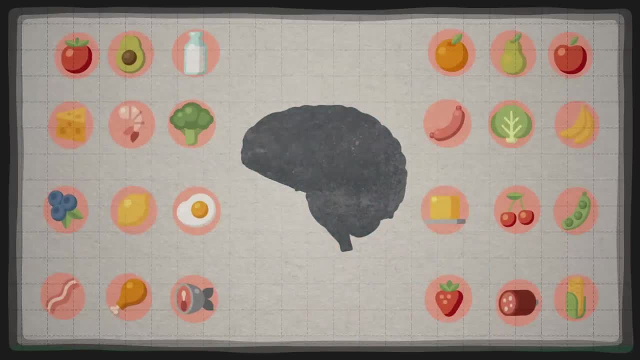 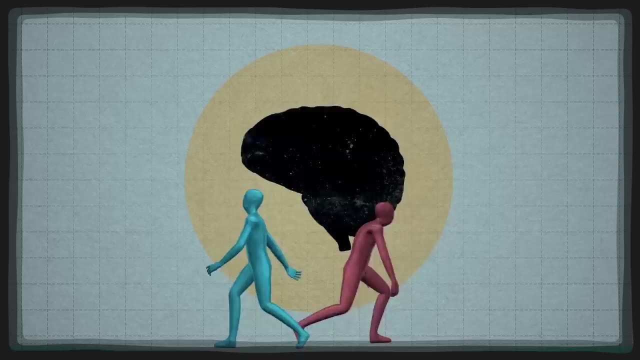 and serotonin, But getting to your brain cells is tricky and amino acids have to compete for limited access. A diet with a range of foods helps maintain a balanced combination of brain messengers and keeps your mood from getting skewed in one direction or the other. 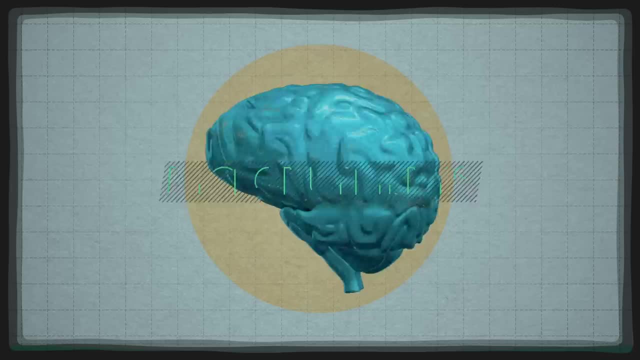 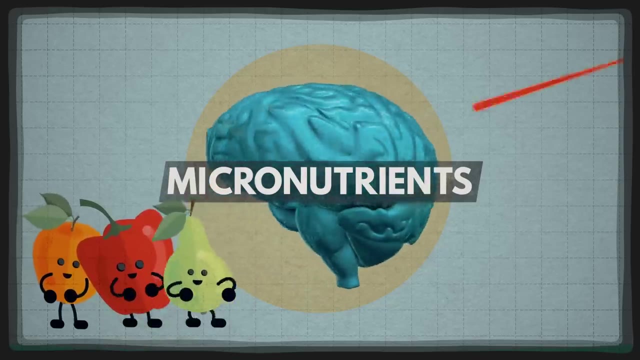 Like the other organs in our bodies, our brains also benefit from a steady supply of micronutrients. Antioxidants in fruits and vegetables strengthen the brain to fight off free radicals that destroy brain cells, enabling your brain to work well for a longer period of time. 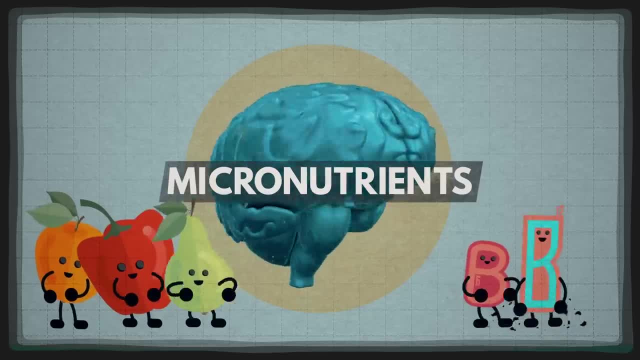 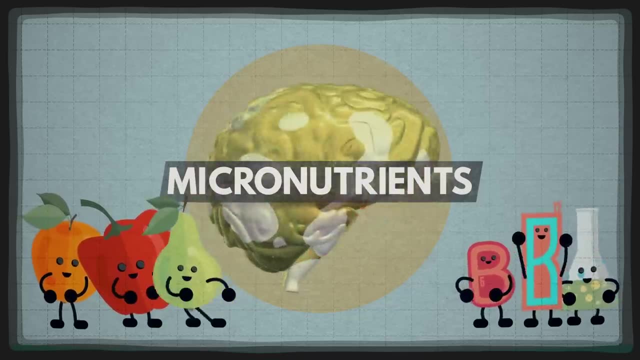 And without powerful micronutrients like the vitamins B6,, B12, and folic acid, our brains would be susceptible to brain disease and mental decline. Trace amounts of the minerals- iron, copper, zinc and sodium- are also fundamental to brain health. 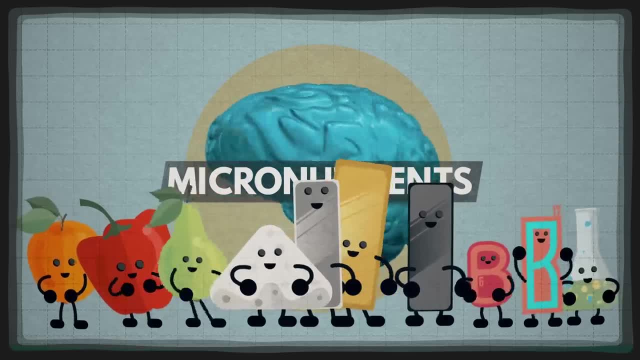 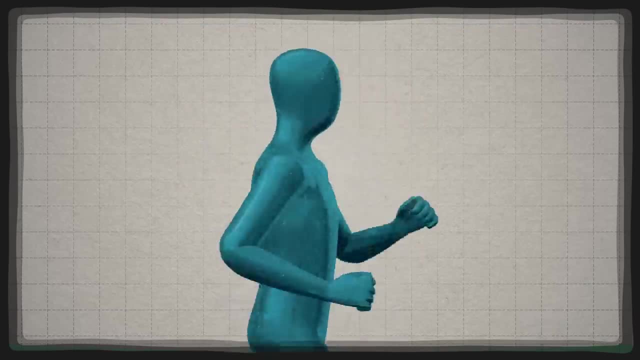 and are also fundamental to brain health and mental health and early cognitive development. In order for the brain to efficiently transform and synthesize these valuable nutrients, it needs fuel, and lots of it, While the human brain only makes up about 2% of our body weight. 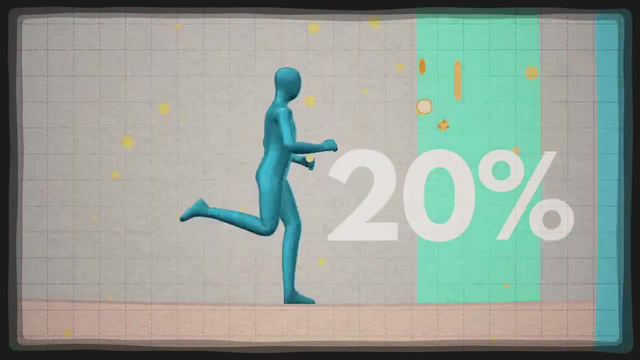 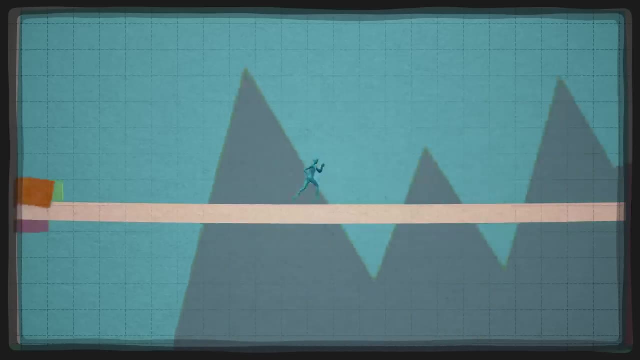 it uses up to 20% of our energy resources. Most of this energy comes from carbohydrates that our body digests into glucose or blood sugar. The frontal lobes are so sensitive to drops in glucose, in fact, that a change in mental function 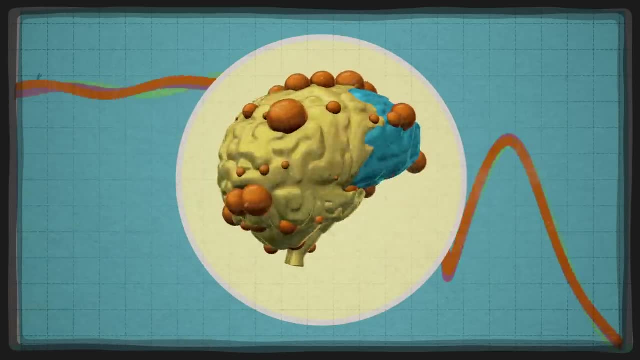 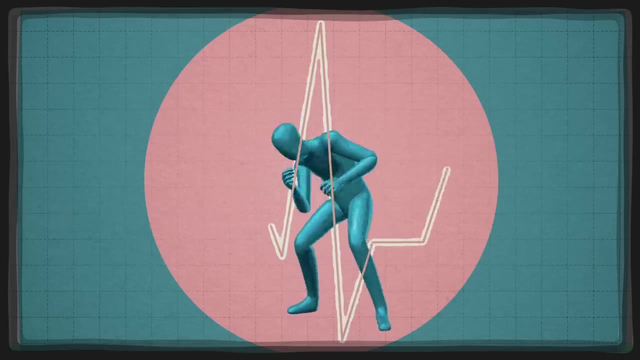 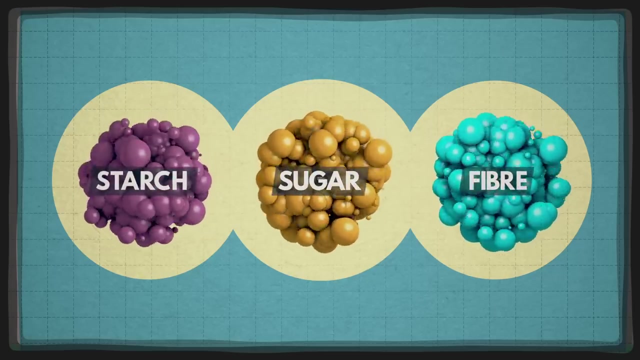 is one of the primary signals of nutrient deficiency. Assuming that we are getting glucose regularly, how does the specific type of carbohydrates we eat affect our brains? Carbs come in three forms: starch, sugar and fiber. While on most nutrition labels